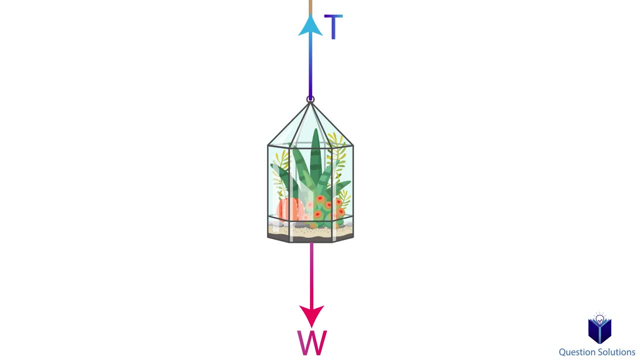 opposite force, in other words a tension in the rope that's holding it in place. Now imagine we have an object like this and there are a bunch of forces and moments affecting it. If we sum up all the forces and moments meaning, we find the resultant force and the couple moment. 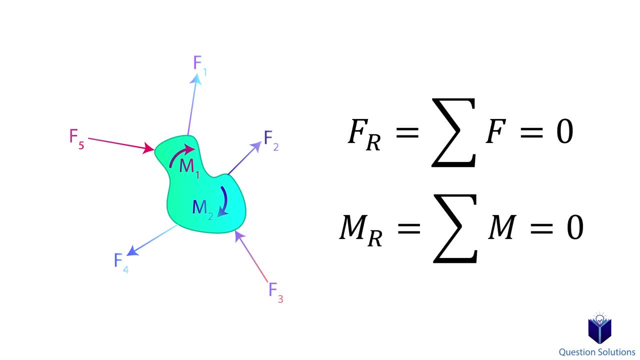 and they're both equal to zero, then that object is in equilibrium. In simple terms, the object is not moving, So this equation means that the sum of all the forces acting on the object is equal to zero. We can break this equation down to forces in the x direction. 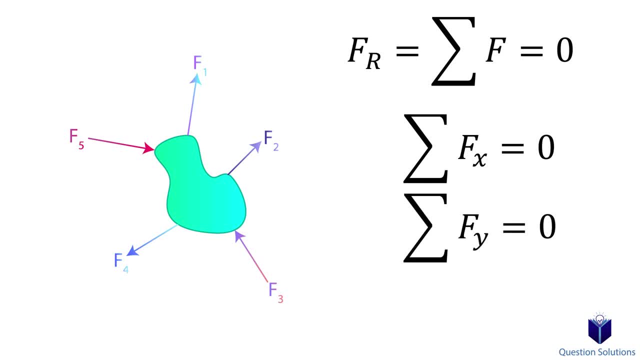 and y direction. So all the forces in the x direction added together must equal zero, and the same for the y-axis forces. This equation means the sum of all the moments – including the ones being applied and the ones being created by the forces – is equal to zero. 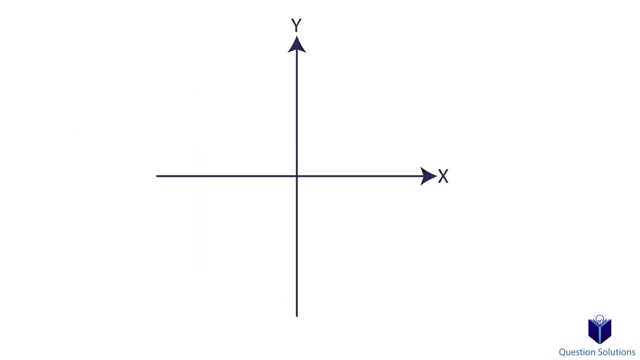 Today we're going to look at just two-dimensional problems, so just objects in the x-y plane. When we look at an object we need to look at something called support reactions. These reactions at the supports are the forces and couple moments that keep an object from moving. 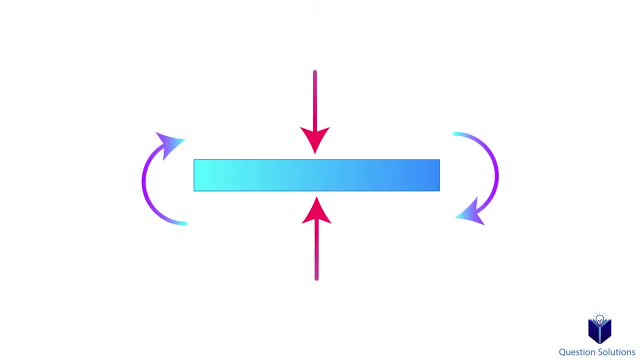 They create opposite forces and moments so that an object doesn't translate or rotate. So in our flower pot example, the rope is a support reaction. The rope is a support reaction. It creates the tension which keeps the flower pot from falling. Let's explore more support reactions. 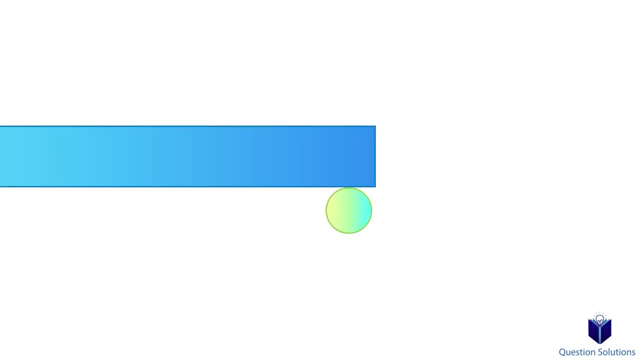 Here we have a bar. There are two support reactions: One is a roller and the other is a pin. Let's focus on just the roller first. Assume that our object can move and we apply a force from the left, Notice how our bar moves. That's because a roller can only prevent vertical movement. 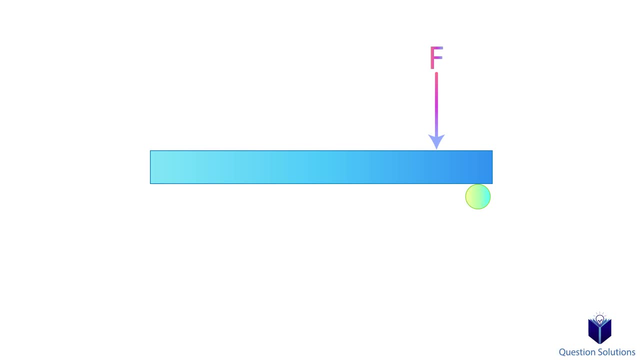 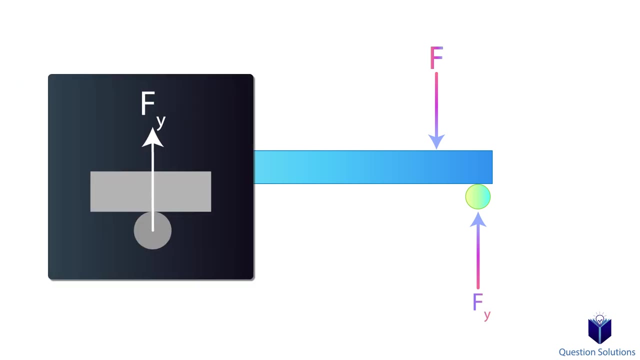 If we apply a force from the top, the roller prevents the bar from moving down by creating an opposite force. So if we're given an object with a roller as a support, that roller can only exert a vertical force which prevents the object from translating in the vertical direction. 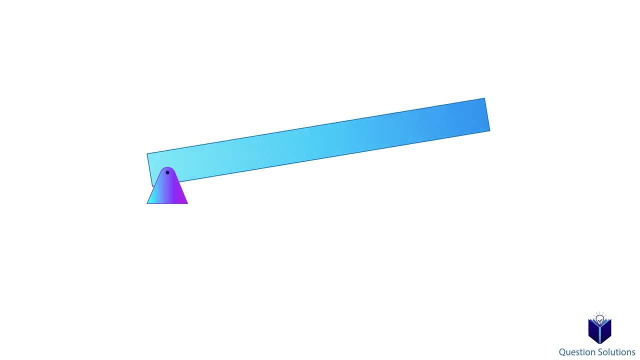 Now let's take a look at the pin side. With a pin the bar can rotate, but it can't move vertically or horizontally. So that means at a pin it would exert two forces, One in the x direction and another in the y direction. 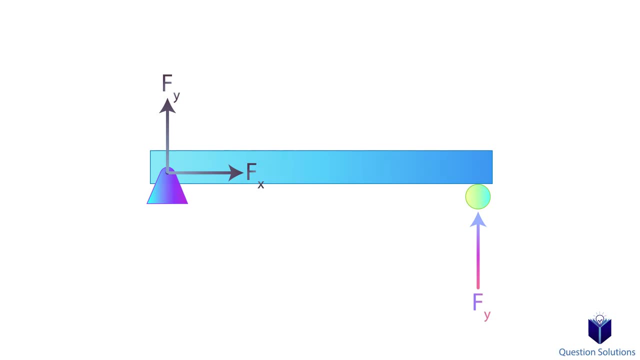 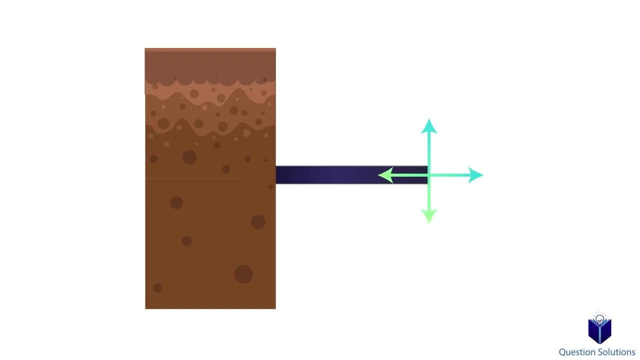 In all of the supports we just looked at, rotation can occur. However, imagine we fix our beam to the ground Or to a wall. Now it can't move in the horizontal direction or the vertical direction, and it also cannot rotate. In this case we'd have two reactions. 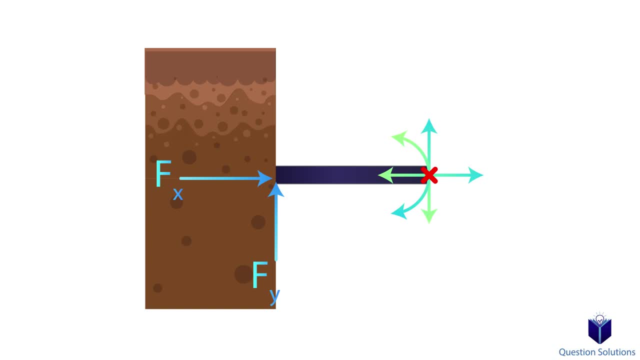 One in the x axis and another in the y axis, And we would also have a couple moment, because rotation cannot occur. In other words, an opposite couple moment must be developed so that the bar doesn't rotate due to the moments created by the forces. 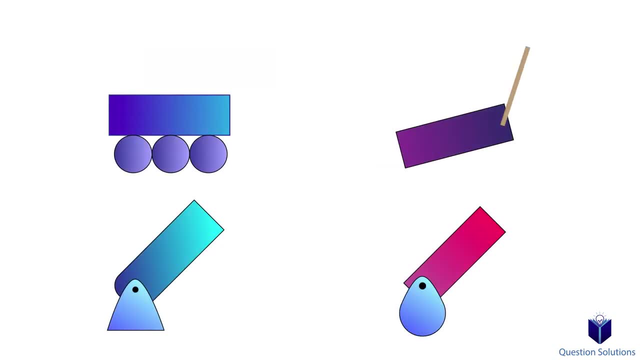 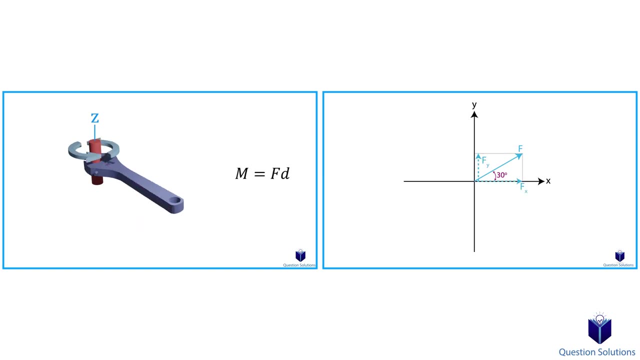 Your textbooks will contain a list of these supports and what type of reactions they can have, So please take a look at those. Lastly, to solve the problems you face, you must know how to break forces into components and how to figure out moments created by forces. 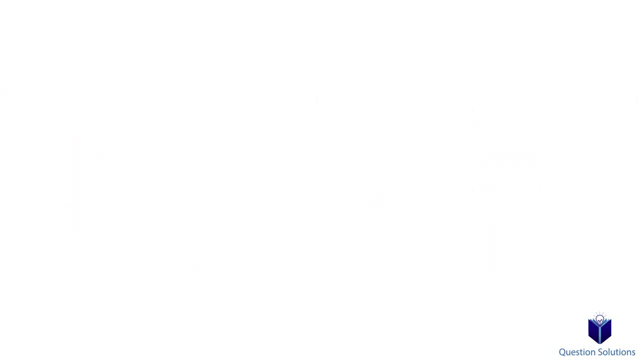 If you don't remember or need a refresh, please check the description. Now let's get to some examples and see how we can actually solve for unknown reactions. Let's take a look at this problem where we need to find the reactions at pin A. 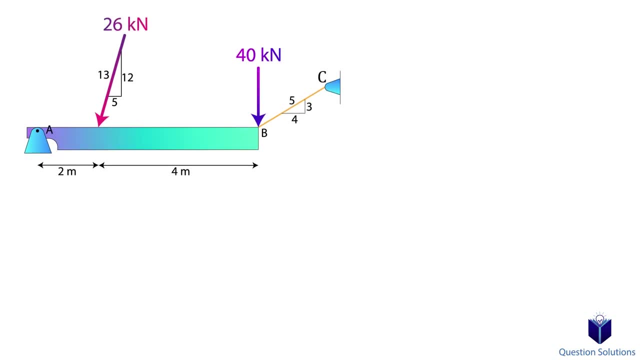 and the tension in the rope. The first step is to draw a free body diagram. Since we have a pin at A, we know there will be two reactions: Ax and Ay. Next we look at the forces. in our diagram We have a 26kN force and we draw it broken into its x and y components. 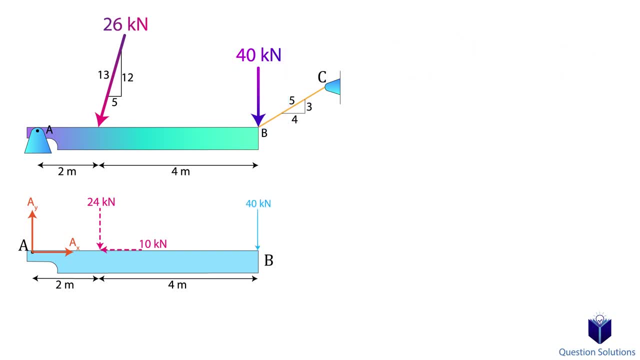 Then we have a 40kN force straight down. Lastly, we have the tension in the rope, which can also be broken into its x and y components. Now it's time for us to write our equations of equilibrium. First, we will consider the x-axis forces. 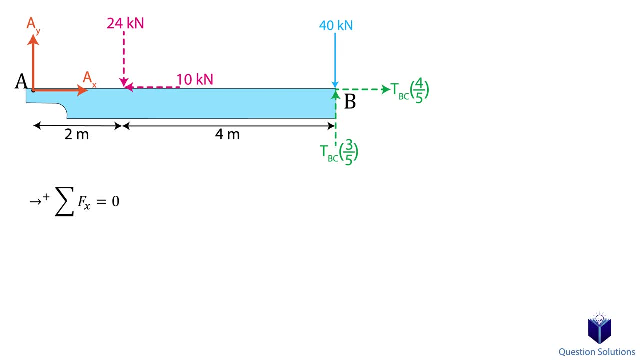 So what we are saying here is that for this object to stay in equilibrium, the sum of all the forces in the x direction must be equal. We will assume right to be positive. So we have Ax, then we have the 10kN force, but notice, it's negative. 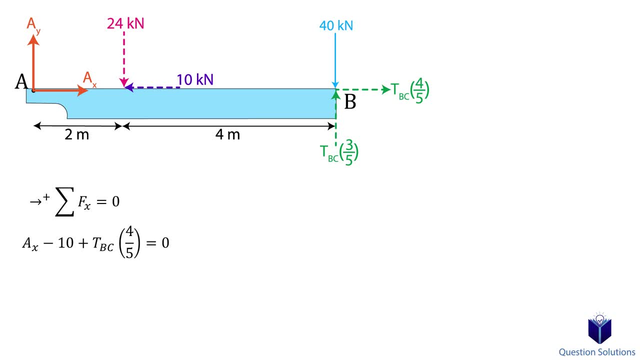 That's because we assume right to be positive and our force is facing left. Lastly, we have the x-component of the tension in the rope. All of this added together is equal to zero. Next, an equation for the y-axis forces: We will assume up to be positive. 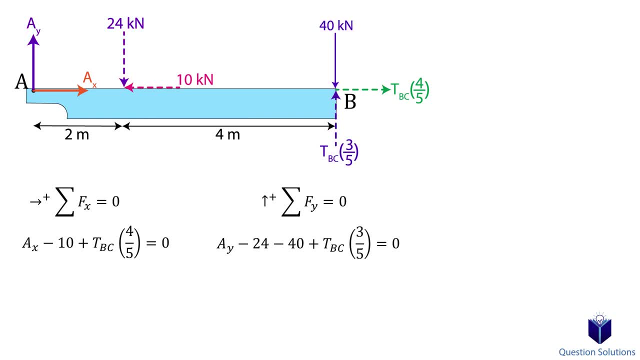 It's the same as before, but now we're just looking at vertical forces. Now we have two equations, so we have the x-axis and the vertical forces. Now we have two equations with three unknowns. So that means we need one more equation and that's going to be a moment equation. 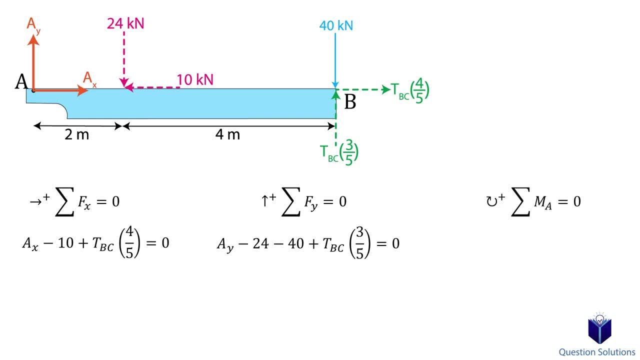 This is usually the case with most questions. You will end up needing three equations: One for the x-axis forces, one for the y-axis forces and then one moment equation. We want to eliminate as many unknowns as possible, so we're going to write our moment equation above point A, which gets rid of Ax and Ay. 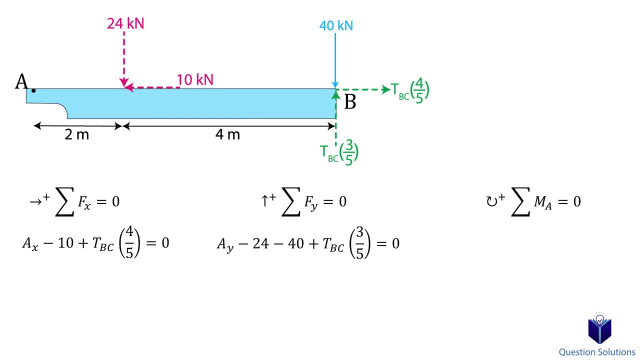 Remember, wherever we calculate the moment about, we ignore the forces applied at that point because they're line-of-factor. So, for example, if we picked point B, then we ignore the forces at point B. Now we will pick clockwise to be positive and write our moment equation above point A. 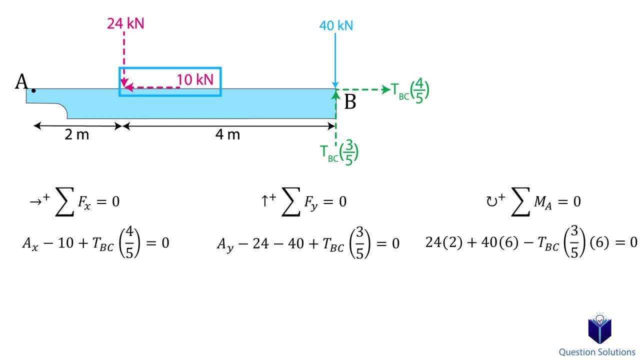 The 10kN force, which is our x-component, won't create a moment, and that's because its line-of-action goes through point A. The same goes for the x-component of the tension in the cable, So only the y-components create moments. 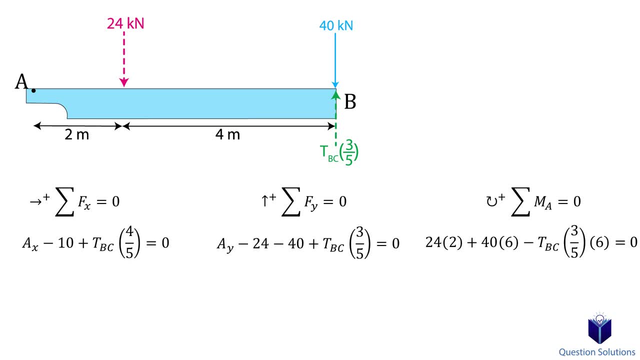 With this we now have three equations with three unknowns, so you can solve them easily. Solving gives us the reactions at pin A and the tension in the cable. Notice that we got a negative value for Ax. All it means is that it's opposite to the direction we assumed. 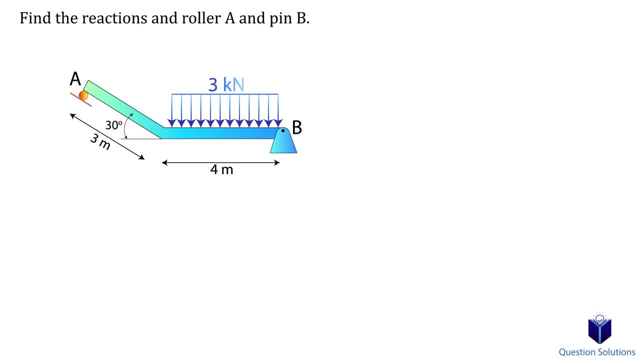 Let's take a look at this problem, where we need to find the reactions at roller A and pin B. The first step is to draw a free-body diagram. Since it's a roller, at A it will only have a vertical reaction. At B, we will have both x and y reactions. 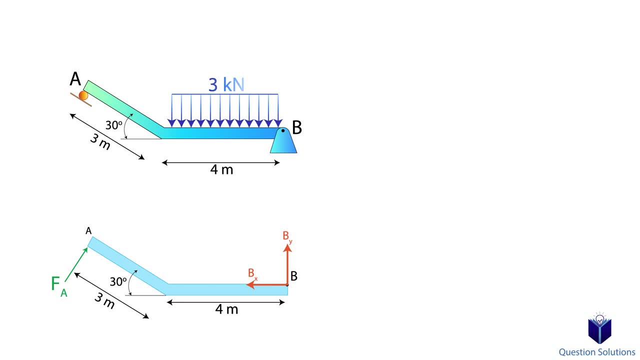 The distributive load has to be expressed as a resultant force, which can be found by multiplying the load by the length, and that gives us 12kN. And it will be placed at the center, so two meters away from point B. 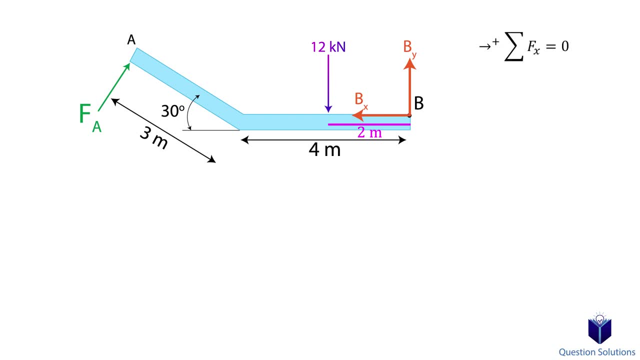 Now we can write our equations of equilibrium. First, the x-axis forces. Note that the reaction at A is at an angle of 30 degrees, so we can break it into x and y components. Next, the y-axis forces. We see that we have two equations with three unknowns. 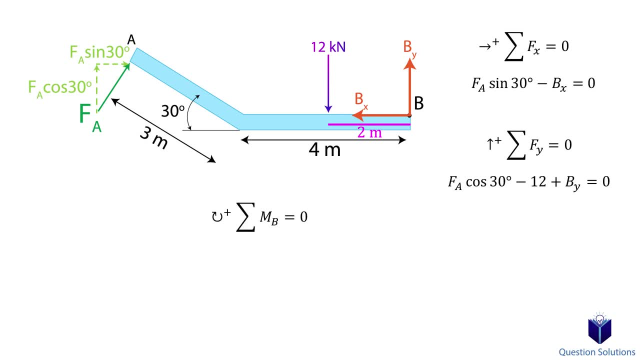 so we need one more equation, which will be a moment equation about point B. We pick point B because there are two unknowns there and we always want to get rid of as many unknowns as possible. We will assume, clockwise, to be positive. 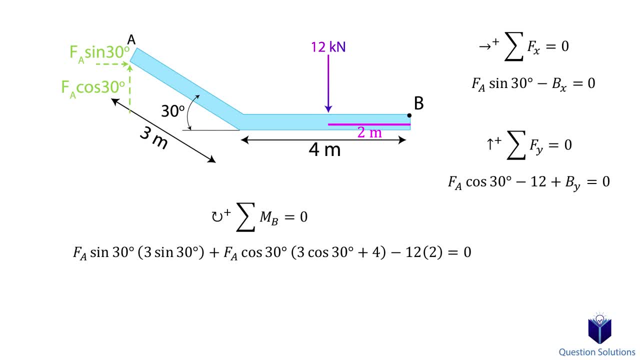 Focusing on the force at A, we have two components. Both will create a moment. For the x component, we have a perpendicular distance of 3 sine 30 degrees. For the y component, we have 4 meters plus 3 cos 30 degrees. 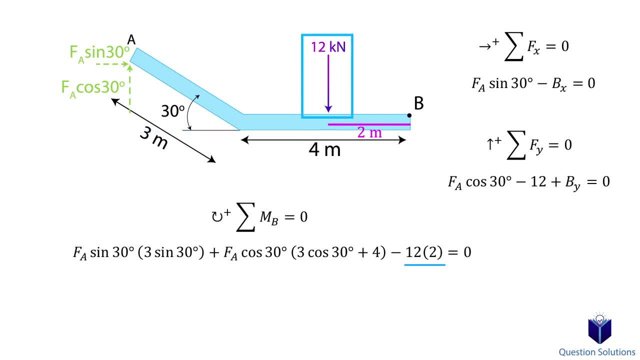 The only other force is the 12 kN force, which is 2 meters away from point B. We now have three equations with three unknowns. Solving gives us the reactions at A and B. In this question we need to figure out the reactions at A and at B. 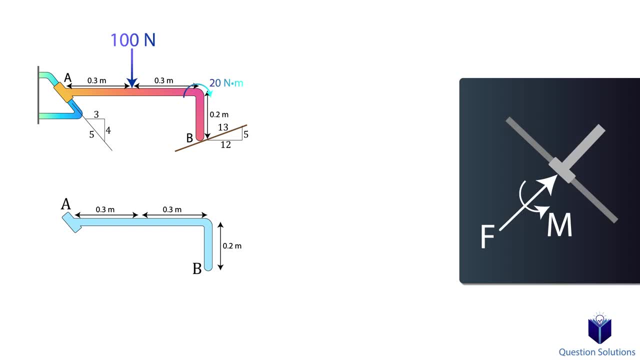 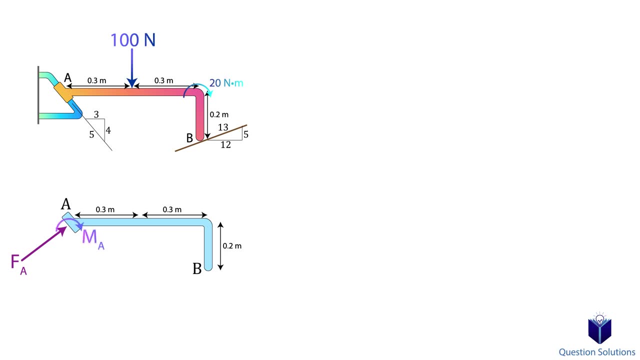 Let's draw a free body diagram. At A we see that it's a smooth collar. so that means it will have a force perpendicular to the rod And there's also going to be a moment created about A. At point B, which is a smooth contacting surface, we will have a reaction force that acts perpendicular. 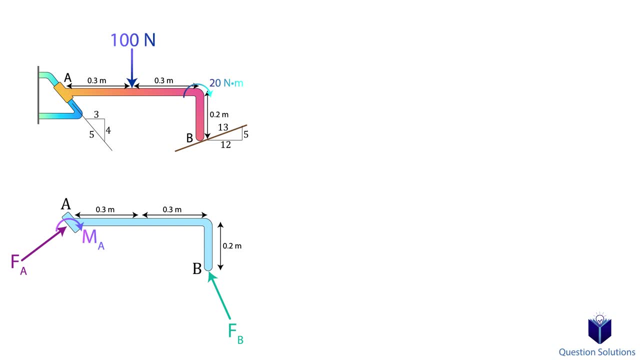 to the surface. Since the forces are perpendicular, all that happens is that the given ratio triangles just flip. There is also a 100 N force. that's straight down, and we also have a moment of 20 Nm applied at the bend. 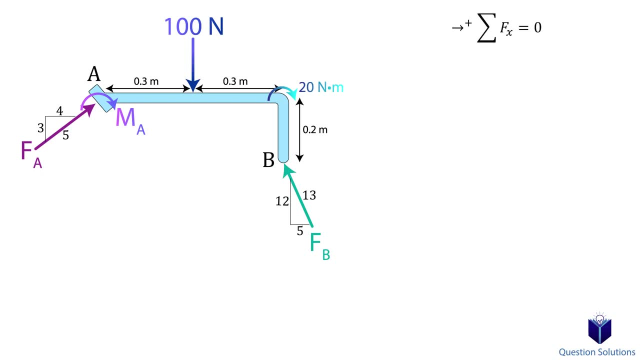 Now we're going to write our equations of equilibrium. Let's start with an equation for the x-axis forces. Note that we're using the x components of the forces. Next, an equation for the y-axis forces. From these two equations we can solve for forces F and F. 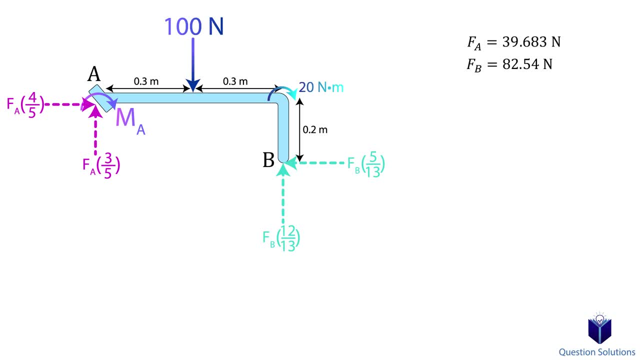 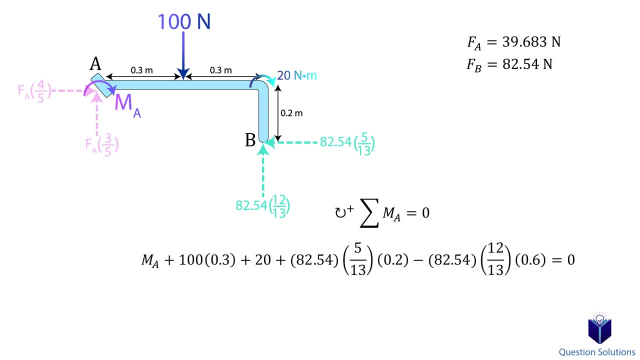 Now We need to figure out the moment created about the smooth collar. For that we can write a moment equation about point A and we will assume, clockwise, to be positive. So at A the reactions at A are ignored because their line of action goes through point A. 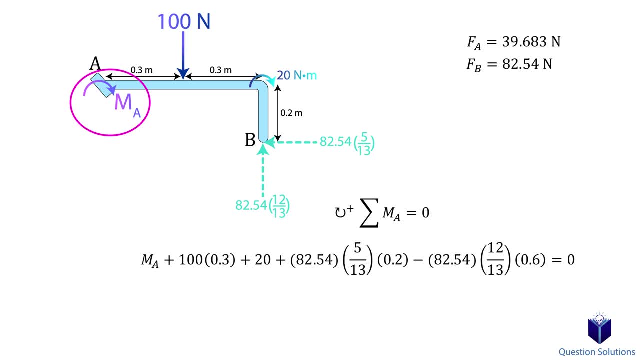 However, we still need to consider the moment about point A. That moment must be included in our equation. Next, we have the 100 N force and the perpendicular distance is 0.3 meters. After that, we have the 20 Nm moment applied at the bend. 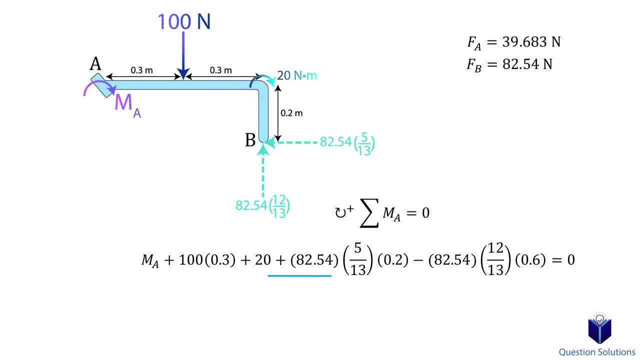 And it's a clockwise moment, so it'll be positive. Finally, we have the x and y components of our force at B. For the x component, the perpendicular distance is 0.2 meters and for the y component it's. 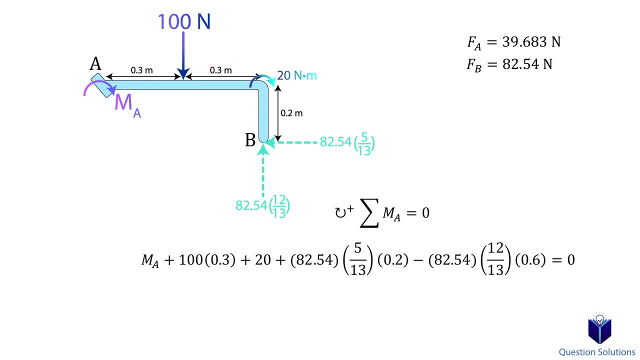 0.6 meters. The x component creates a clockwise moment and the y component creates a counterclockwise moment. Solving gives us the moment at A, but notice that it's a negative value. All it means is that the moment is opposite to our assumption, so it's actually counterclockwise. 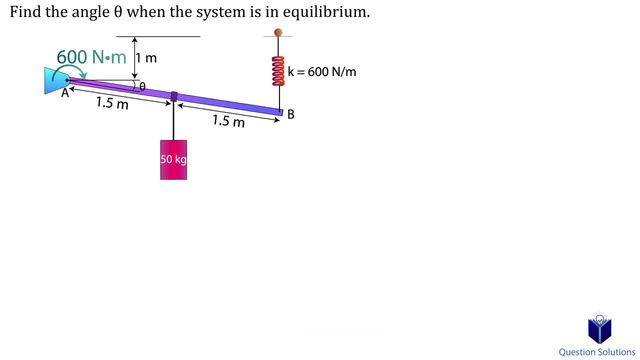 The moment is actually counterclockwise. Let's take a look at one last example. In this example we have a weight attached to a rod and on one end it's pinned and at the other end we have a spring. 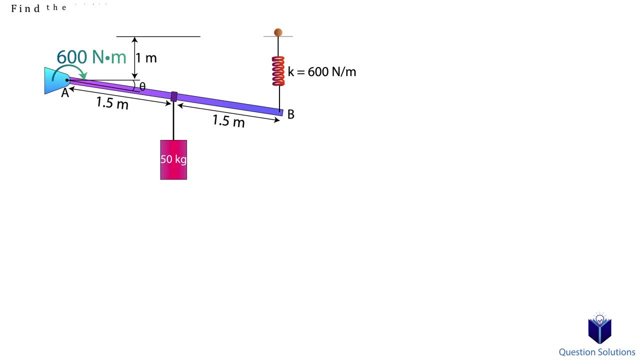 We need to figure out the angle created when the system is in equilibrium. First we have to draw a free body diagram. At pin A we have two reactions. We also have the moment applied at A. Note that this moment is not created about pin. 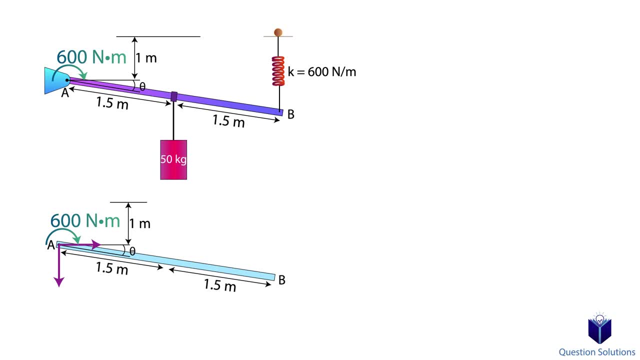 A by other forces. It is something that was manually applied. Now we look at the weight of the cylinder. It's mass times the acceleration due to gravity. Here the angle that's created at this point is the same angle that's created here, because 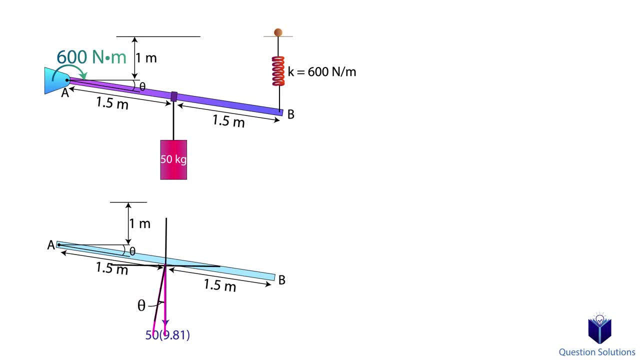 if we place our coordinate system like this and move it, you can see that it'd be the same. Lastly, we have the force of the spring that's straight upwards. Now we have to put on our thinking caps. So initially, the spring has an unstretched length of 1 meter. 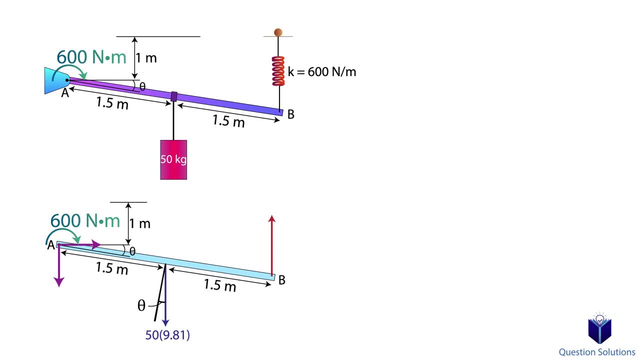 In the second state, when everything moved, the spring stretched a bit. How much did it stretch? Well, let's draw a right-angle triangle. Let's draw a right-angle triangle. Let's draw a right-angle triangle like this. Notice how the length of the stretch is the opposite side. 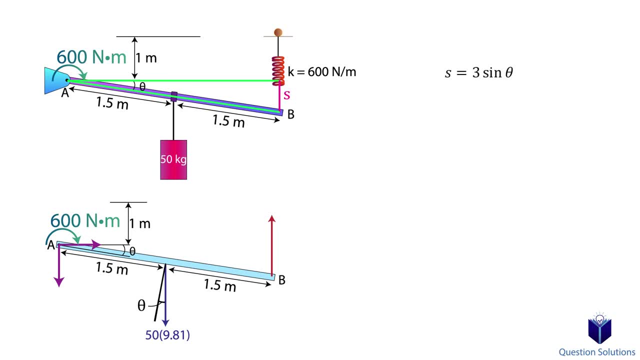 So we can use sine to figure it out. Now what we've found is the length this spring stretched. So to find the force, we use Hooke's law. The stiffness is 600 newtons per meter. Let's simplify Now. also notice that when we draw this force, the angle that it creates is once again the. 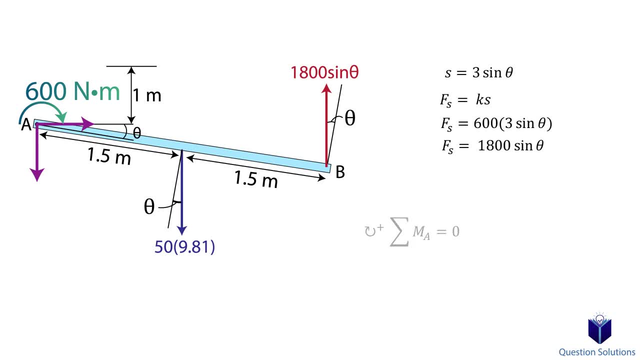 same. Finally, we can figure out the angle. In fact, we actually only need a single moment equation about point A. That would get rid of the force. Finally, we can figure out the angle. In fact, we actually only need a single moment equation about point A. 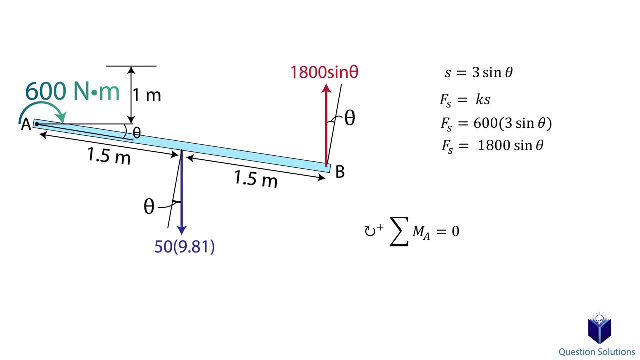 That would get rid of the force. Finally, we can figure out the angle That would get rid of the force. Finally, we can figure out the angle That would get rid of the force. Finally, we can figure out the angle. 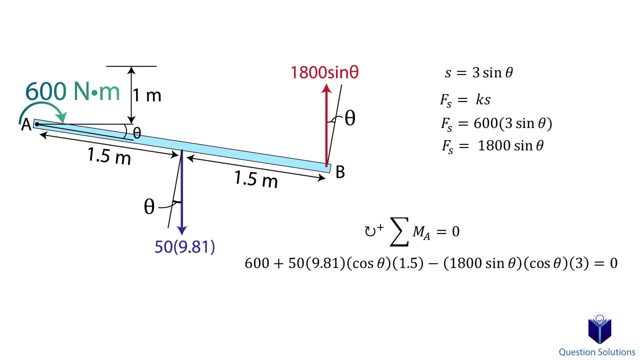 That would get rid of the force. That would get rid of the two unknown reactions and only leave the angle to be found, because we know all the other forces. That would get rid of the two unknown reactions and only leave the angle to be found, because